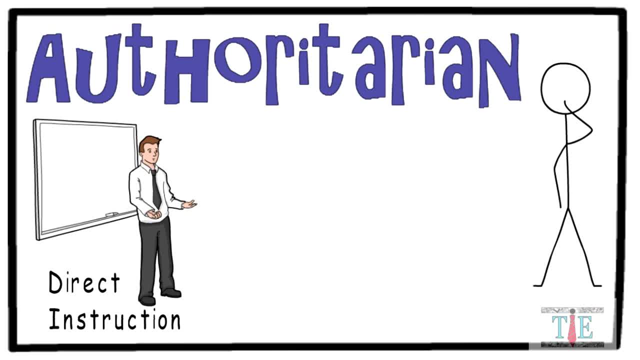 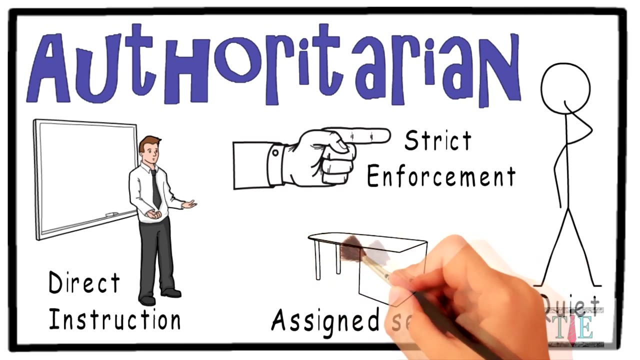 The student says The authoritarian style teacher does not want to take any questions from the students In this classroom. classroom rules are strictly enforced. The teacher is very firm and unflexible when it comes to the rules. Authoritarian teachers like to have their students sit in assigned seats for the entirety of the year. These teachers are very organized and like to see their students in one place. 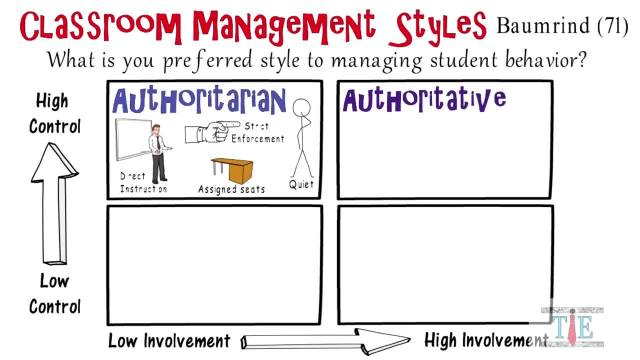 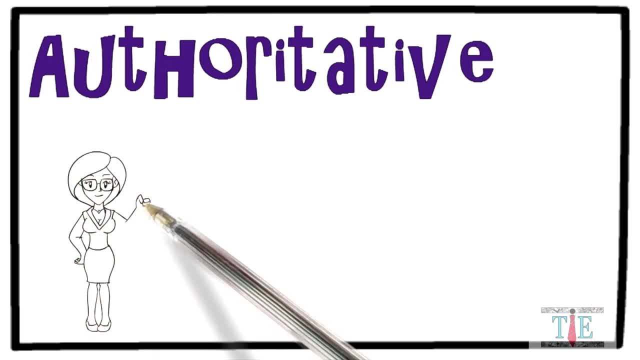 Next up the authoritative teacher, Teachers with high control and highly involved in their students. The authoritative teacher enforces their rules but also hears the students out. These teachers are both firm but also fair to their students. The authoritative style looks to give students their own voice. Classroom discussions are encouraged. 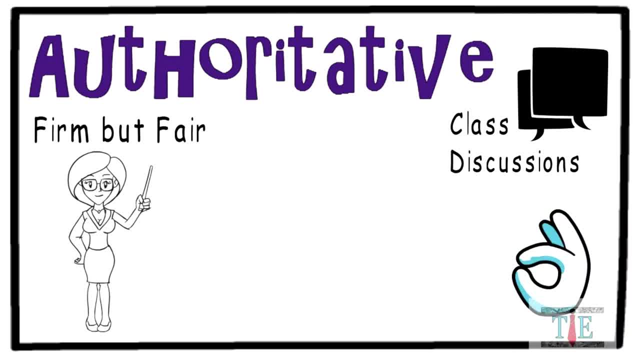 This teacher cares a great deal about their students. The teacher wants to see their students succeed and you often see a lot of positive feedback from the teacher, From the teacher. These teachers consider the consequences of their actions—authoritative teachers carefully weigh the circumstances of a student's inappropriate behavior. 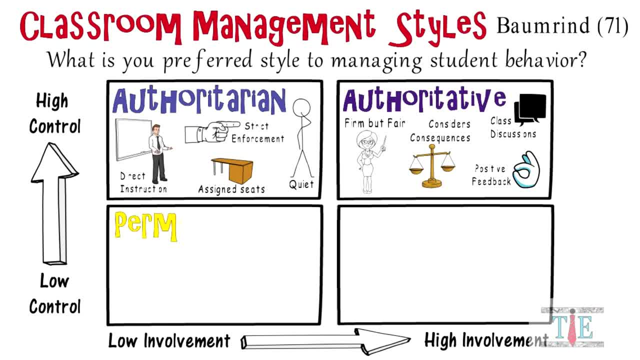 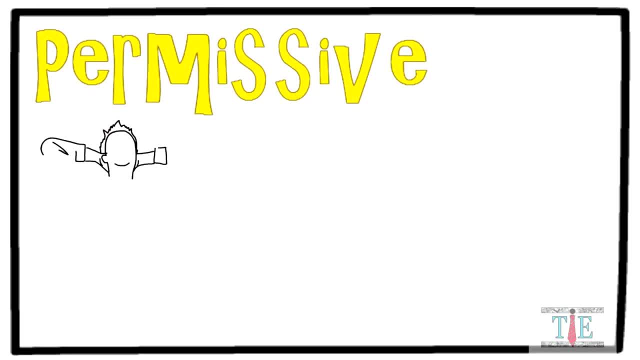 Next up the permissive style—very little control and very little student involvement. Unfortunately, this is a teacher that doesn't really care about their teaching career. Teaching is just a way to pay the bills. The permissive teacher often doesn't take the time to prepare lesson plans. 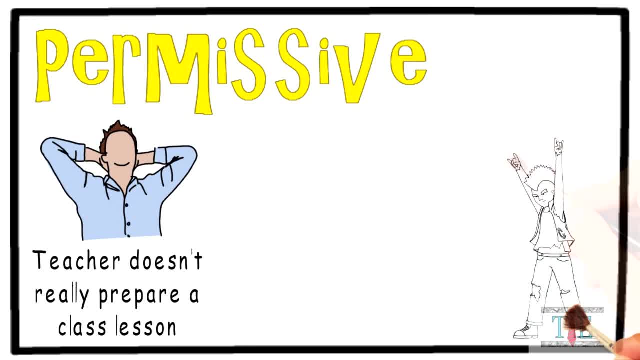 Permissive-style classrooms are out of control. Students are out of their seats doing whatever they please. A teacher doesn't take the time to go over classroom rules or procedures. Permissive teachers often show movies during class time. They do this simply because they do not feel like teaching. 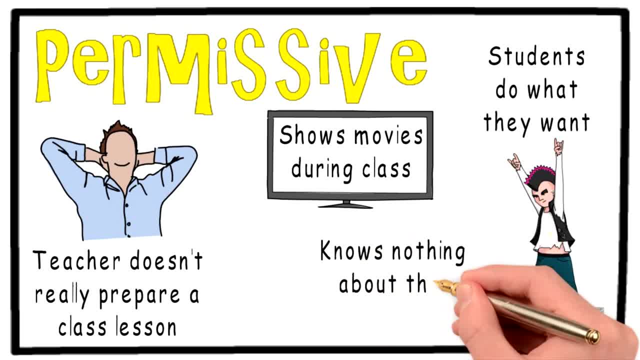 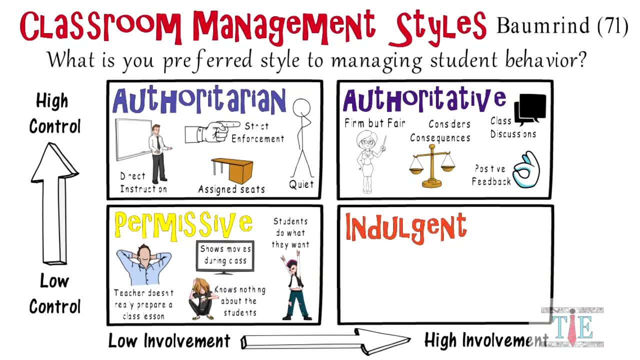 The permissive teacher doesn't know much about his students. He doesn't care about the kids. Teacher-student relationships are of little importance to him. Permissive teachers don't notice suffering students And, lastly, indulgent. Very little control but highly involved in the students. 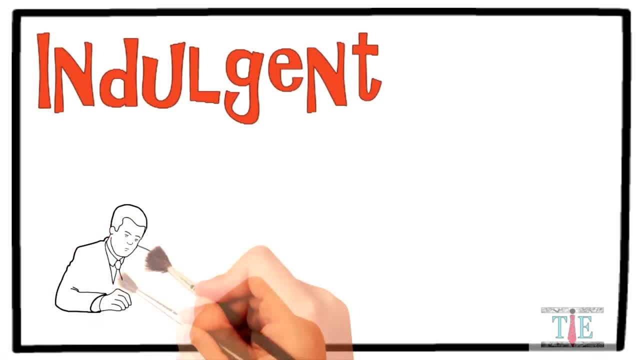 The indulgent teacher takes their career as a teacher very seriously. They work very hard to plan fun and exciting lessons. You can count on this teacher to come to class prepared. The indulgent style of classroom management believes in a student-empowered learning model.